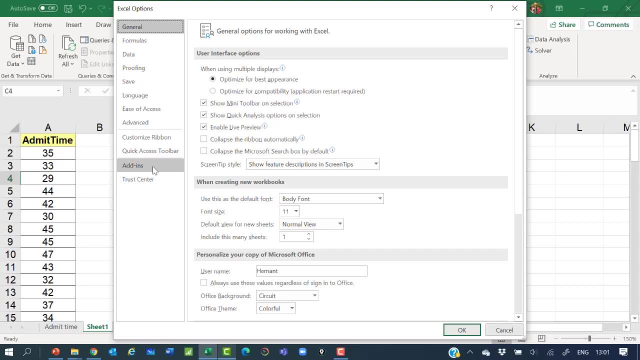 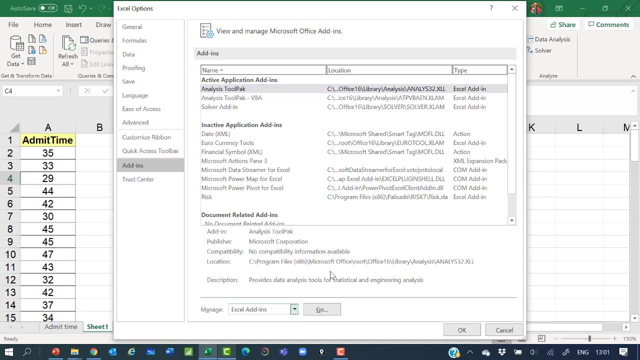 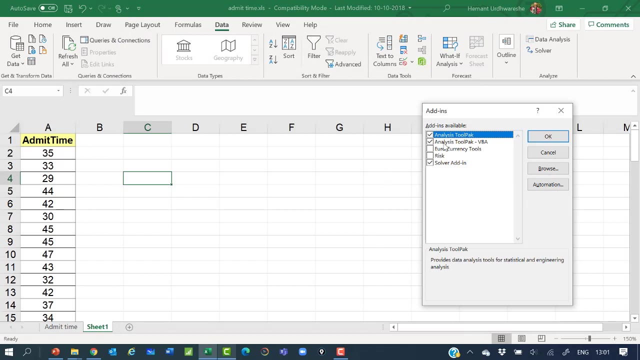 and select the add-ins and then select the analysis tool pack. Once you click there, click on the go button and you will see the choice there. You will see multiple boxes Out of it. you have to definitely choose the first two boxes, that is, analysis tool pack and tool pack VBA. You. 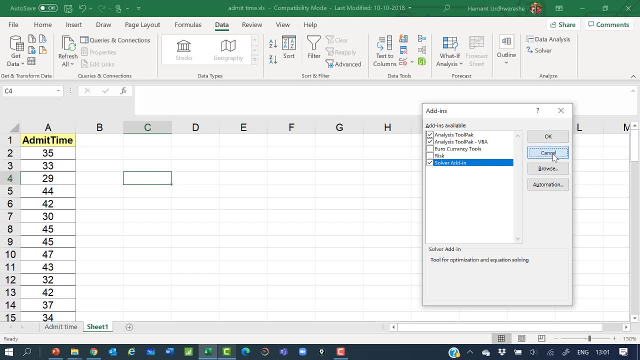 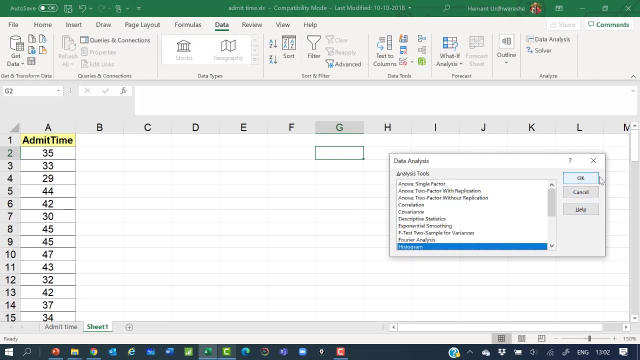 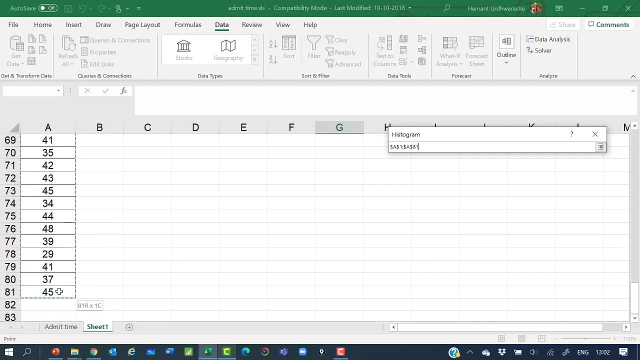 can also choose the solver and click OK. I have already installed it so I'm not pressing OK. So we go back and we go to data, data analysis and histogram command. So click on the data and data analysis histogram And select the data, including the labels, and check the labels box. 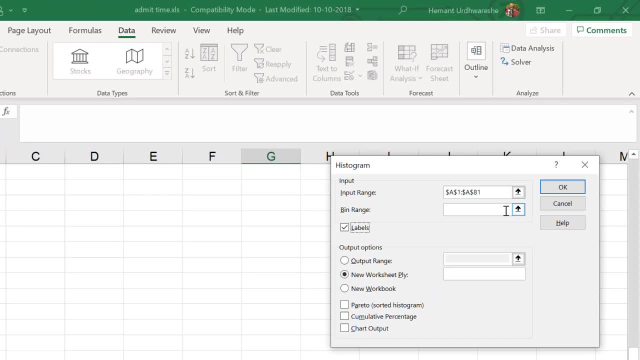 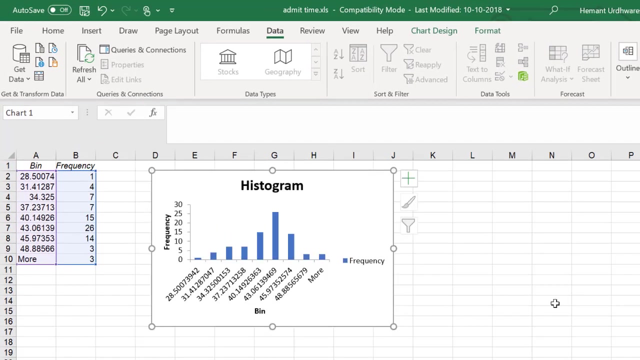 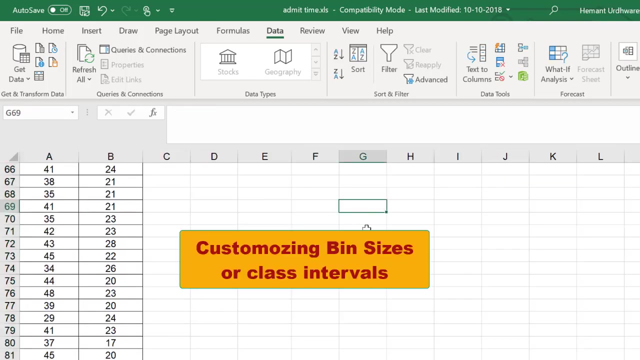 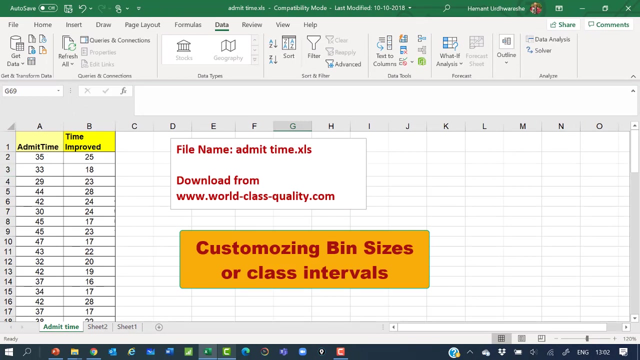 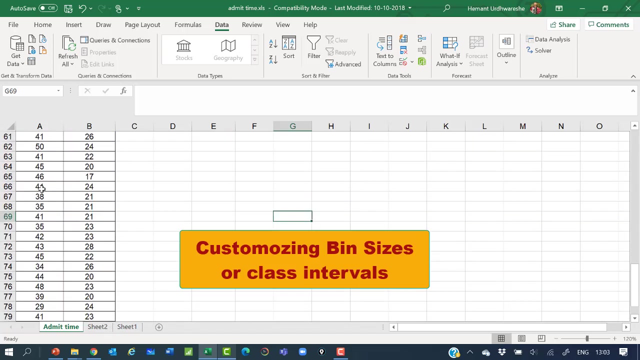 there And you can leave the bins blank and then select the chart option there and click OK. You will immediately see the histogram there. It will be on a separate sheet because you have chosen option of new worksheet. So you see the histogram Now. this histogram may not be with the same bin sizes in your mind, So you may choose to have different bin sizes. If you want to do that, you can. you can observe the minimum and maximum values in the data and choose your own bins. 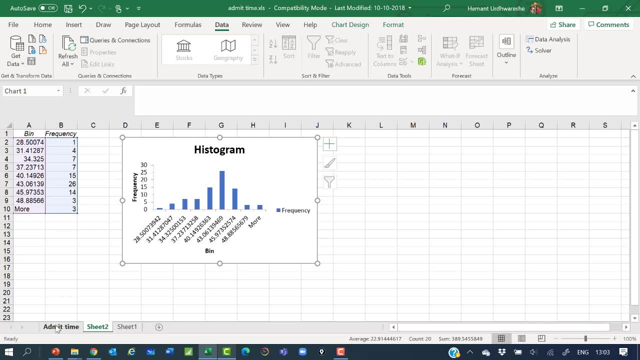 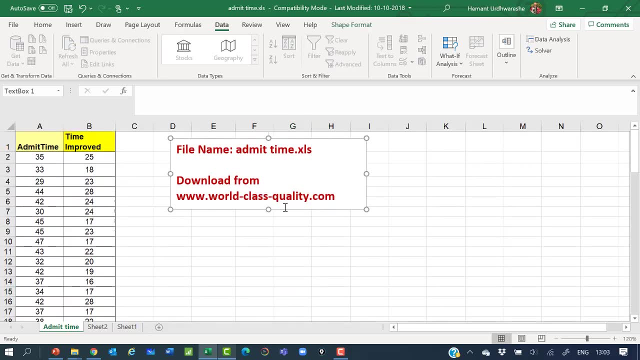 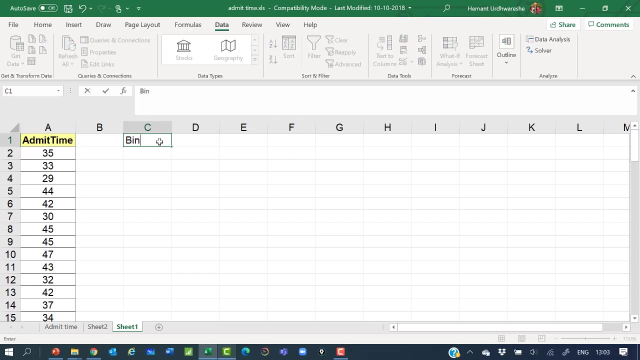 I'm just showing you how to do that. You can also see the previous histogram to see what is the minimum and maximum. And now we go to the again the same worksheet to create the bins. We can just create a column called bin And we can start at 25.. The minimum was about 28.. So we start with 25 and we choose the class interval of 5.. So 25,, 30 and then we can. 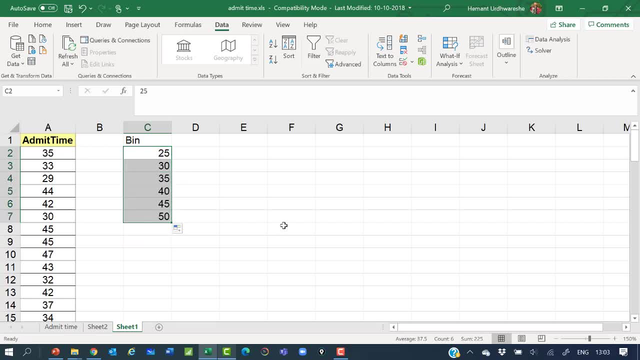 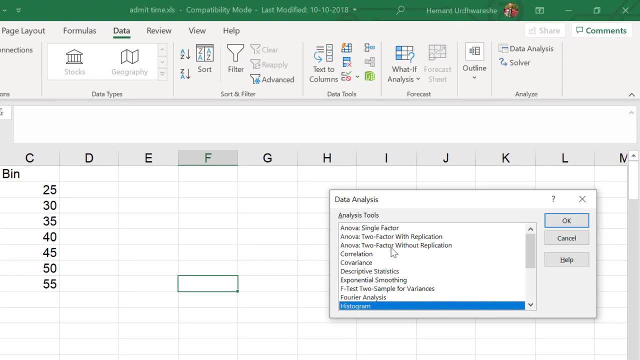 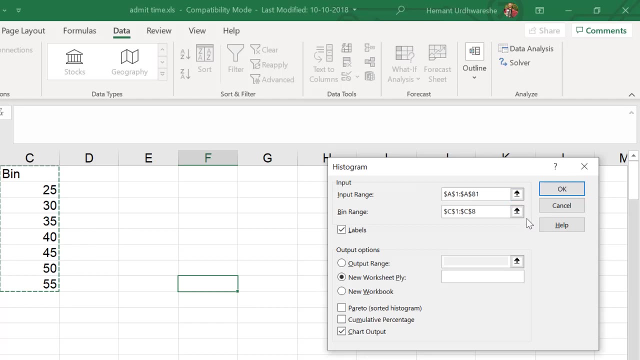 We can have the maximum value of about 55.. Okay, which is probably appropriate, and use the same commands, But now, this time you select the bin Also. so in the bin, Select the bin information And click OK. Now the histogram will again appear in a new worksheet. 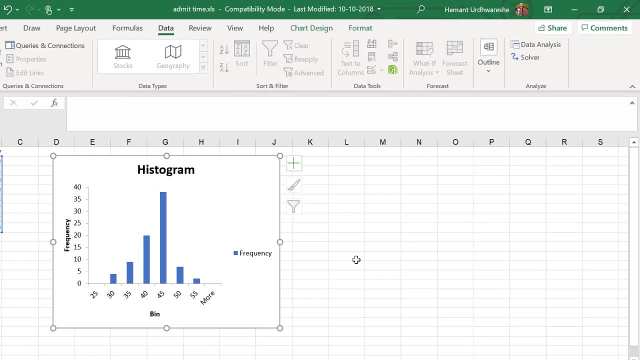 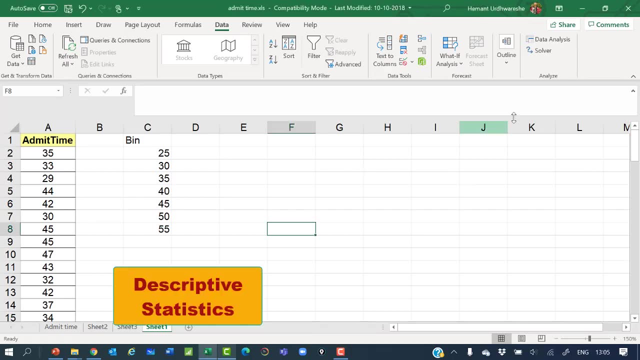 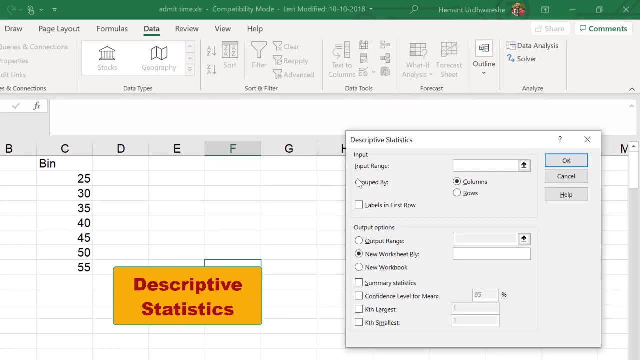 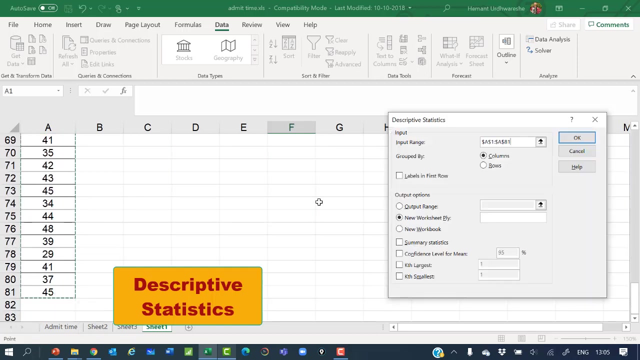 But this time it will be as part of the bins, as part of the been intervals that you have created for your own convenience, the way you want. we can also use the analysis tool pack for for descriptive statistics. so we use the tool pack again, we again select the data. we have selected a descriptive statistics. 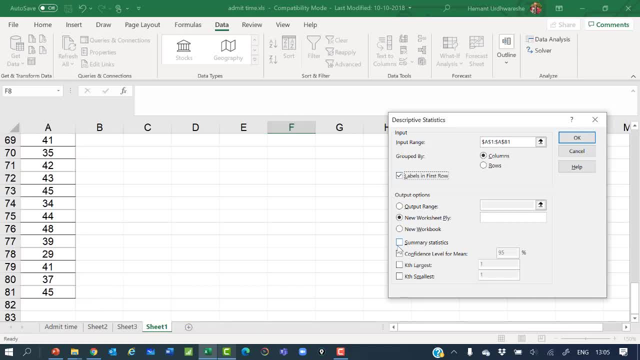 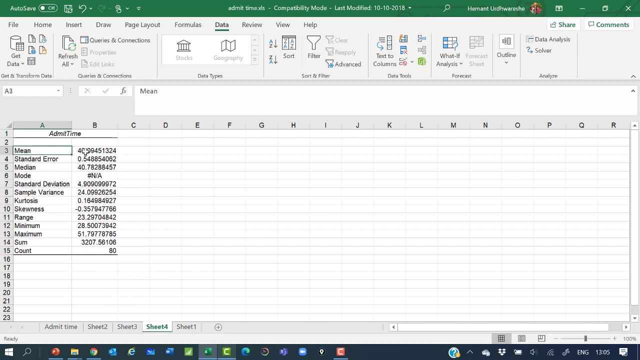 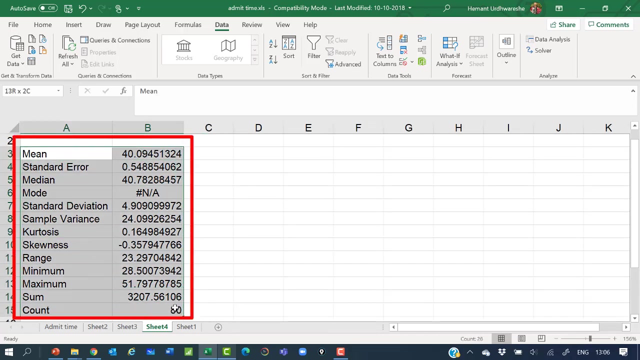 this time. so select the data, choose the labels there, check on the labels and and choose the summary statistics and click ok. then you will see all the descriptive statistics immediately. of course, you have excel commands for everything else, everything that this command uses, but this is a single command that gives you almost everything, so it gives you the mean which. 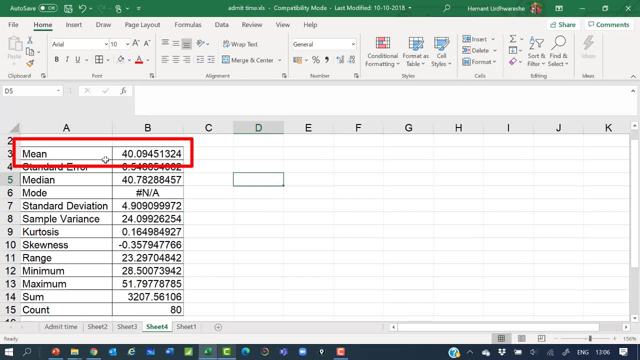 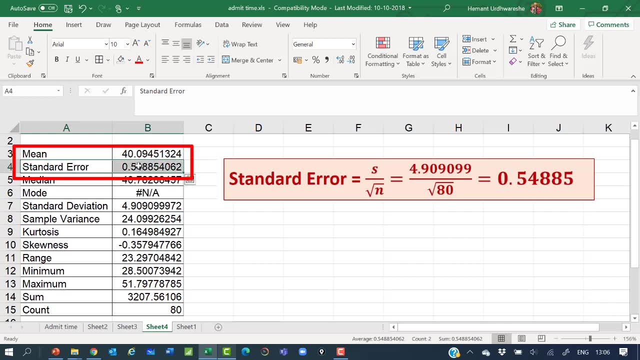 is 40.094 the standard error. we will see what is the standard error. so the mean is 40.094. the standard error is equal to standard deviation upon square root of the sample size and the standard deviation is seen as 4.909. sample variance is square of the standard. 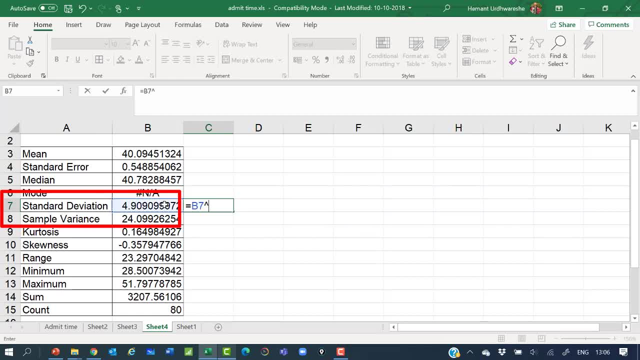 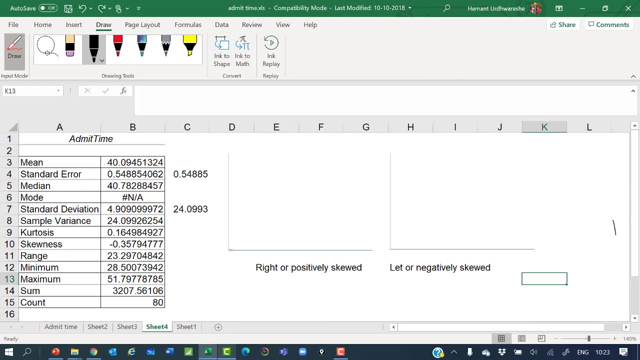 deviation. you can double check that. you can just square the standard deviation and see that the variance equals the sample variance value. then you have kurtosis skewness range: minimum, maximum and the total of all the readings and the count is 80.. positively skewed data has got long right. 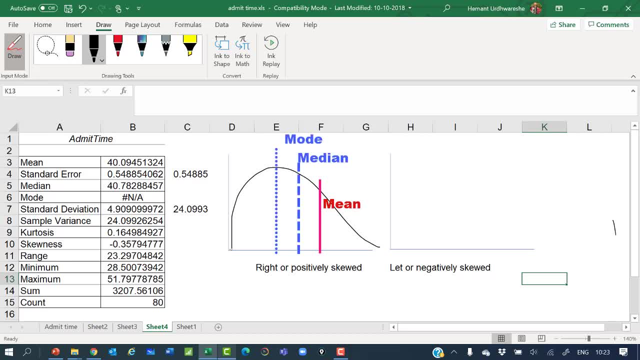 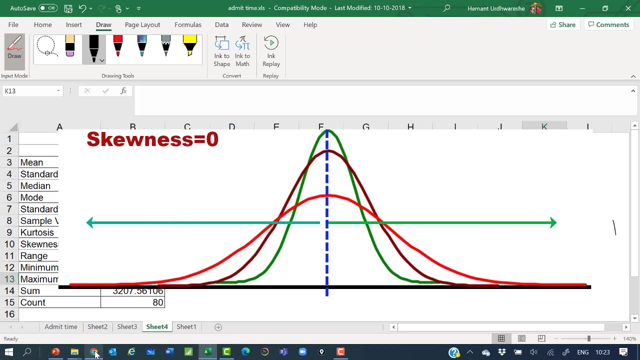 tail and mean is to the right of median and mode. similarly, left skewed data has got long. left tail and mean is to the left of median and mode. for a perfectly symmetric distribution, the skewness value will be 0. in this case, we observe a skewness value of minus 0.3579. therefore, this: 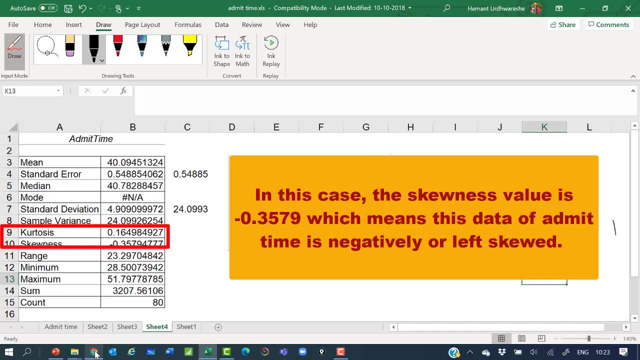 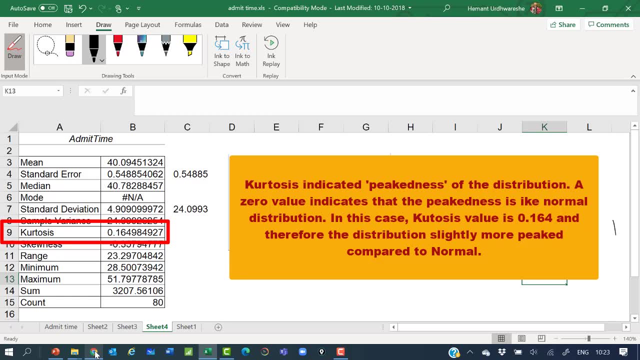 This is negatively skewed distribution. Kurtosis indicates peakedness of the distribution. A zero value of kurtosis indicates that the distribution is like normal distribution. A plus value indicates that the distribution is more peaked compared to the normal distribution. In this case, we observed a kurtosis value of 0.164, which means that the distribution.